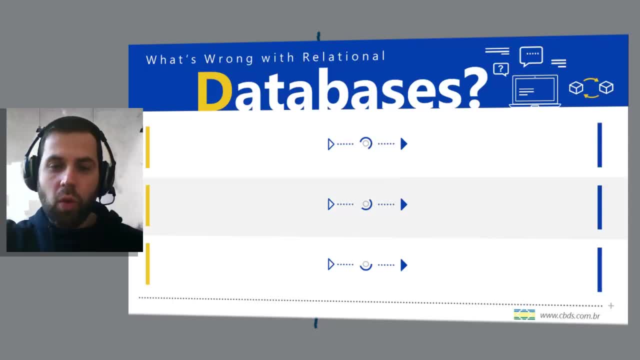 Let's get started this slide with a good question: What's wrong with relational database? It's important to remember a little about history. Every time that a new disruptive technology born is a delicate moment Why You need to learn new terms, think about other approaches that you never thinking before. It's common to have new concepts that are hard to understand, and so on. 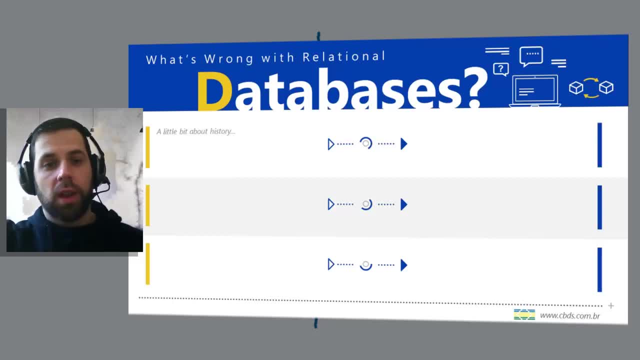 This phenomenon occurs always along the history, When the hierarchical database born in 1966 at IBM, when the relational database born in 70 decades and now recently when NoSQL database come to IBM, into our reality. So really don't worry if you don't understand completely. 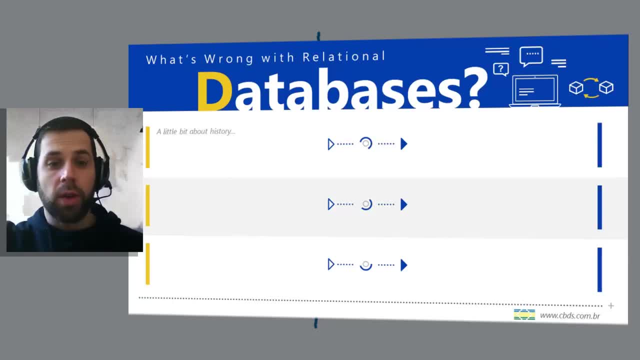 the terms and concepts in a first read about NoSQL database. Our brain is shaped from relational database and this transition is not so easy. Vertical scaling versus horizontal scaling: Nowadays we encounter scalability problems when our relational application becomes successful and usage goes up. 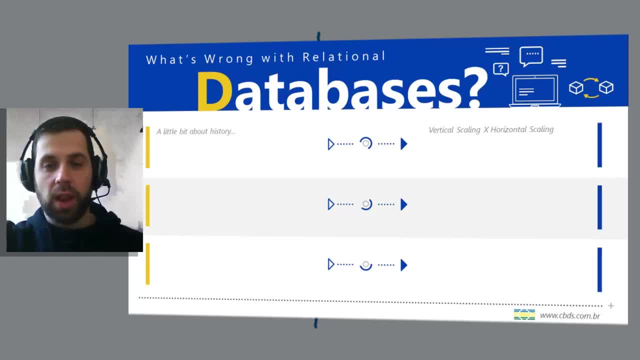 This is a good point. we might consider an alternative to the relational database. When we talk about scalability, we can consider two approaches. One is look in our hardware and put more memory, upgrading disk, put fast processor and so on. This is known as vertical scaling. 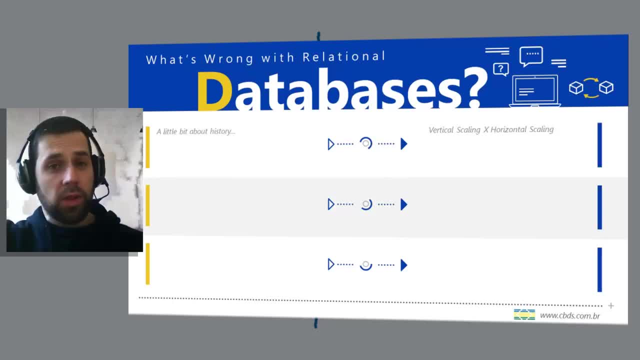 This approach works. Sure, this can relieve you for a time. On the other hand, if you have massive elastic scalability issues, you need to consider the horizontal scaling. What does it mean? One machine, one large machine and a powerful machine. 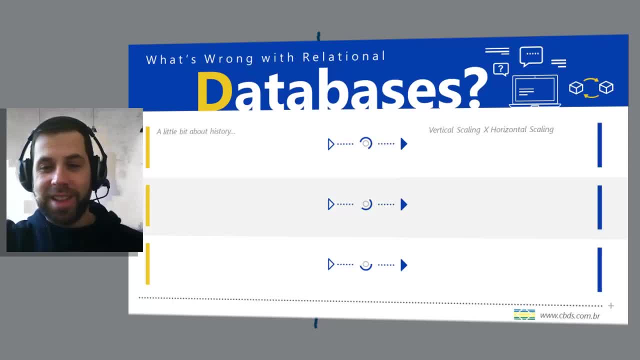 is not enough to solve your problems. You need a 10,, 20, or maybe 1,000 machines to distribute it and solve your problems. If massive elastic scalability is not an issue for you, you need to consider the horizontal scaling. 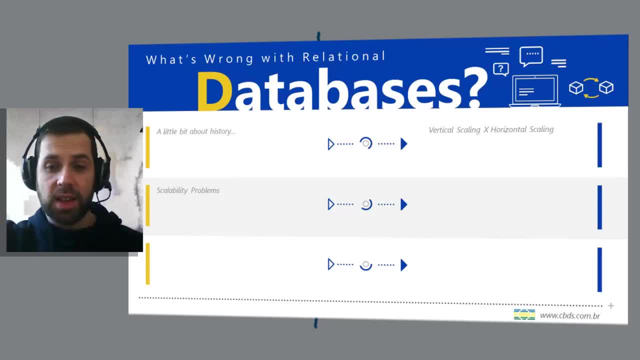 The trade-off is relatively complexity of a system such as Cassandra may be simple, not be worth it. Relational data has served us developers and DBA well, is a fact, but the explosion of the web and in particular social network, means corresponding explosion in the 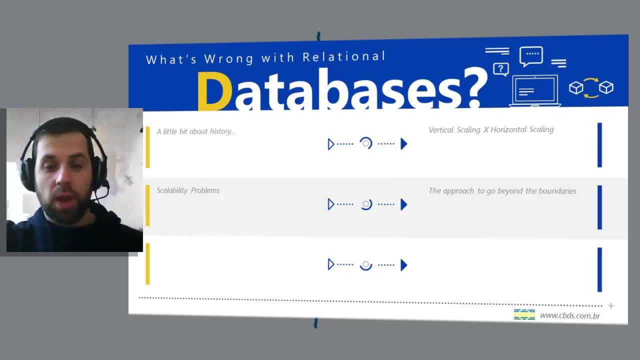 world. We need to think and develop our softwares to go beyond the boundaries And these boundaries. today we are not talking about million records, but billion records. So what problems do you have? I started this slide asking to you what's wrong with relational database. 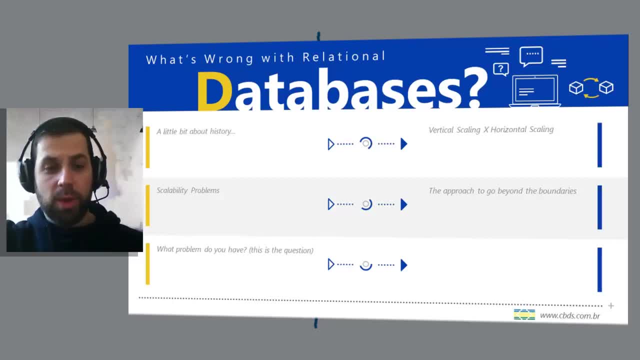 The short answer is nothing. Hierarchical database, relational database, NoSQL database, the horse, the car, the plenty. they each build on prior art. They each attempt to solving certain problems, And so they are each good at certain things and less good at others. 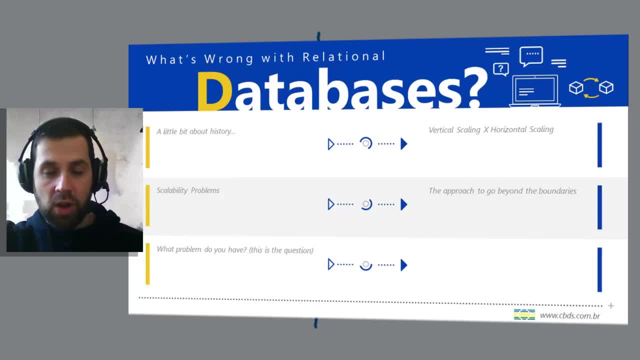 So the real question is: what problems do you have in your applications? You need to ensure that your solution matches the problems that you have, And there are certain problems that relational database solve very well. And last, SQL. One of the most important thing when you talk about relational database is the way of how. 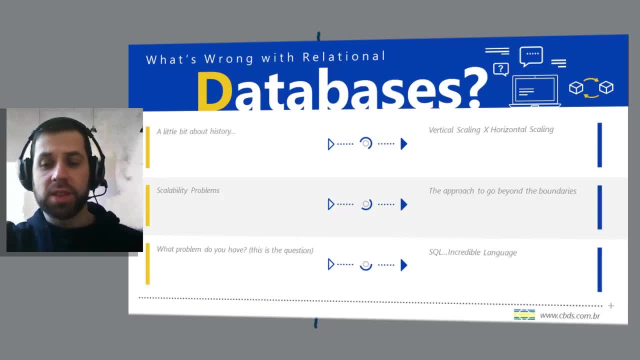 we can interact with the system. SQL is a feature rich and use as simple declarative syntax. SQL is a powerful language. It allows the user to represent complex relationship with the data. You can insert, Select, Delete Or update and merge data. 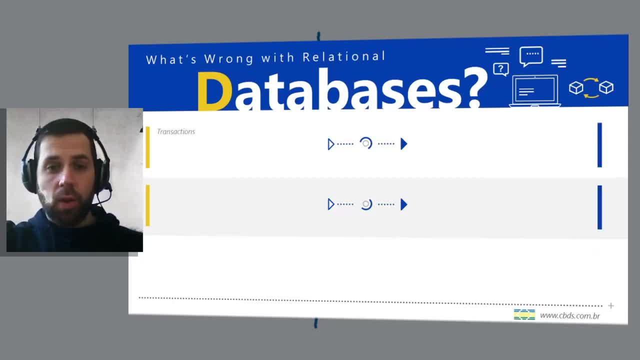 Transactions. Relational database and SQL also support transactions. A database transaction is a transformation state. A key feature of transaction is that they execute virtually at first, allowing the program to undo any changes that may have arrived during execution. ACID is an acronym for Atomic Consistency, Isolated and Durable. 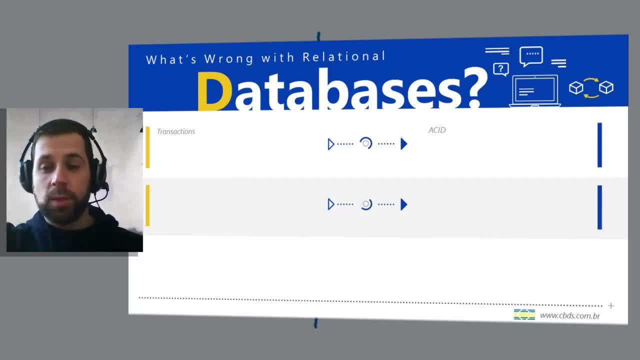 Atomic means all or nothing. That is, when a statement is executed, every update within the transaction must succeed in order to be called successful. Consistent means the data moves from one correct state to another correct state. Isolated means the data moves from one correct state to another correct state. 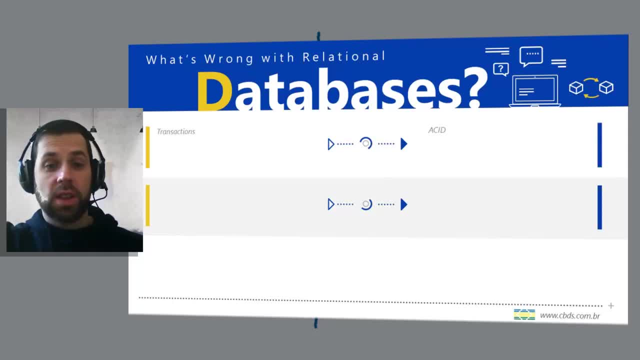 Consistent means the data moves from one correct state to another correct state. Isolated means that transactions executed concurrently will not become entangled with each other's. And last Durable: once a transaction has succeeded, the change will not be lost. 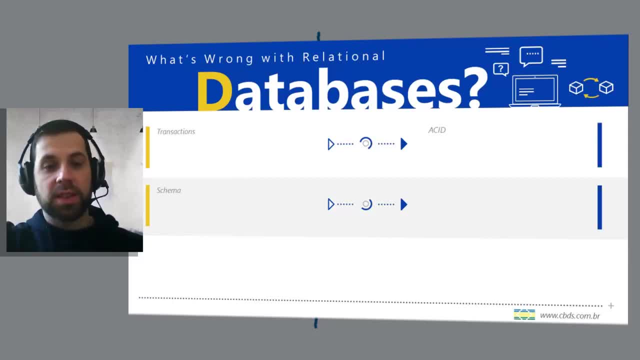 Schema. One feature of relational database system is the rich schema they afford. You can represent your domain objects in a relational model. The intention To create normalized schemas. However, you are sometimes forced to create tables that don't exist as business objects, like the many-to-many tables in your domain. 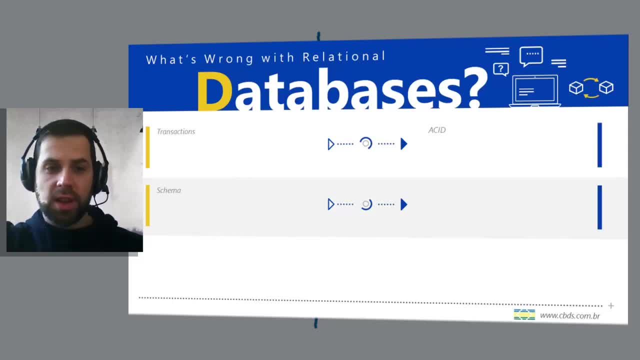 This populates the data model and also forces us to create more complex SQL statements to join these tables together. In a small system it isn't much a problem, But complex queries and multiple joins become a problem. In a small system it isn't much a problem. 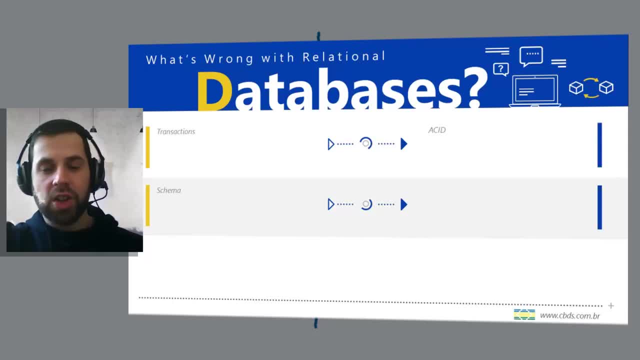 But complex queries and multiple joins become a problem. In a small system it isn't much a problem, But complex queries and multiple joins become a problem. But complex queries and multiple joins become a problem. But complex queries and multiple joins become a problem. 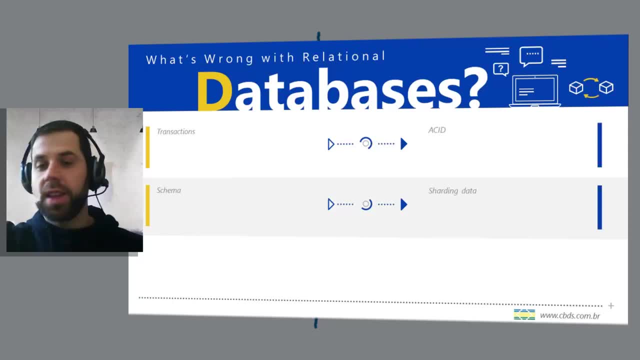 They will become slow once you have a large number of rows in many tables to handle Sharding data. Another way to attempt to scale a relational database is to introduce sharding to your architecture. This has been used to good effect at large websites such as eBay, which support billions. 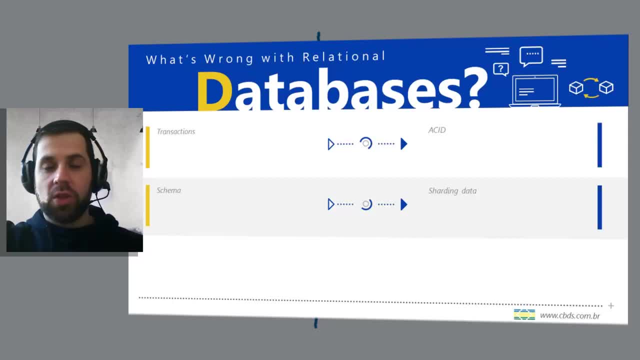 of SQL queries per day and in other Web 2.0 applications. Another feature is Sharding. The idea here is that you split the data so that, instead of hosting all of it on a single server or replicating all of the data on all the servers in a cluster, 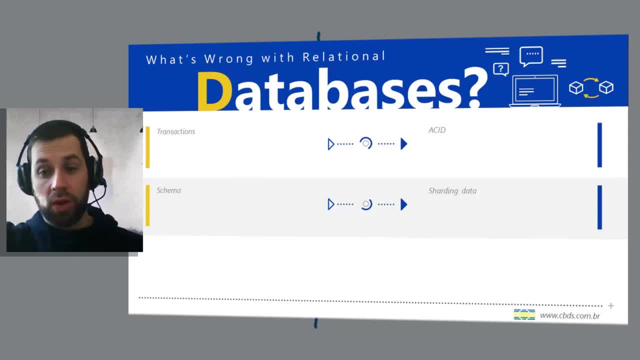 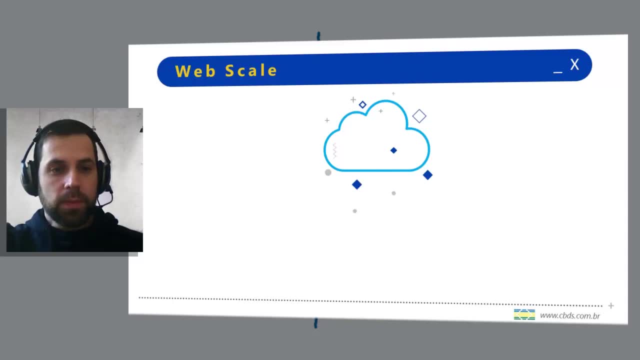 you divide up portions of the data horizontally and host them each separately. Web scale: Let's consider the phenomenal growth about web because, as more and more data becomes available every day, every hour, every second, we need architectures that allow our organizations to take advantage of this data in near time, to support decision-making and to offer new and more powerful features and capabilities to our customers. 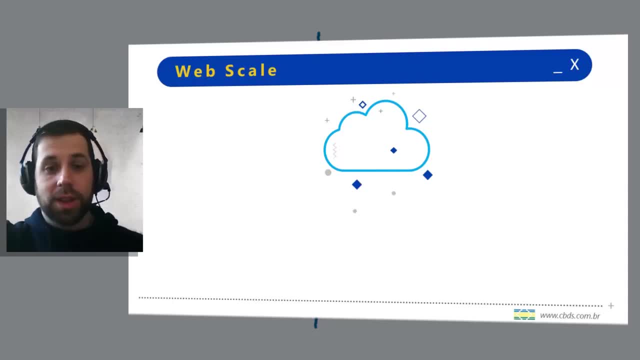 We all know that the web is growing, but let's take a moment to consider some numbers of IDC research paper. YouTube serves almost 5 billion videos every day. Walmart processes over 40 petabytes of data every day. Google recently announced that Gmail has 1 billion active users. 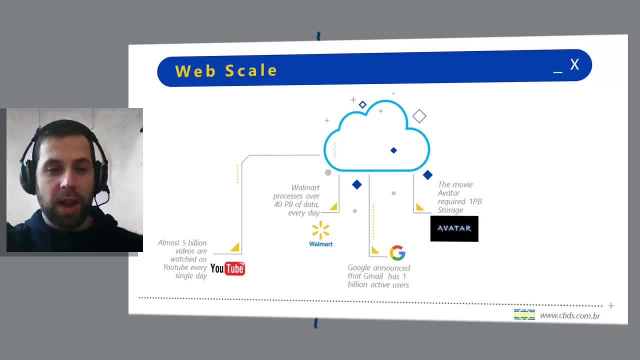 The movie Avatar requires 1 petabyte storage space, or the equivalent of a single mp3 song if that mp3 were 32 years long. The total number of emails account at 2016 is closer to 4.7 billion. 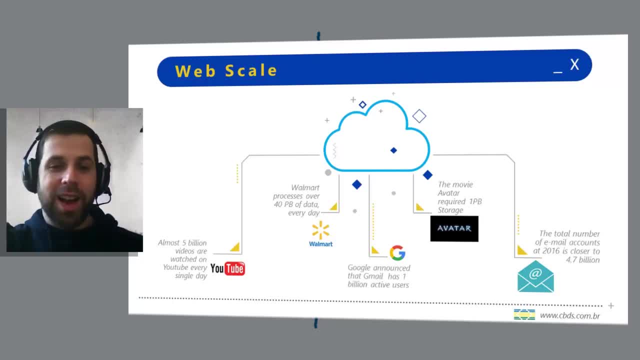 As you can see, there is a great variety of the kinds of the data that are available on the web. As you can see, there is a great variety of the kinds of the data that are available on the web. There is a lot of data that needs to be stored, processes and queries and some variety of the 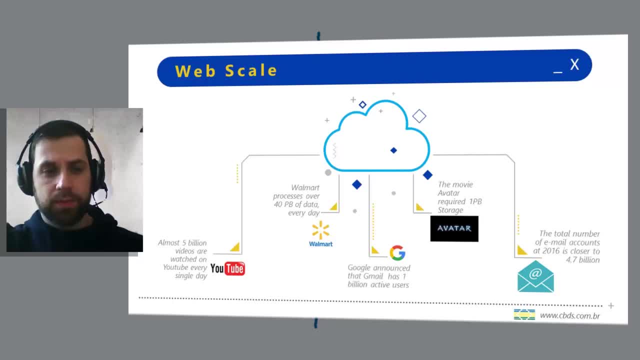 businesses that are using such data. You might then be surprised to learn what, within corporations, around 18% of the data is unstructured. In a world now working at web scale and looking for the future, Apache, Cassandra might be one part. 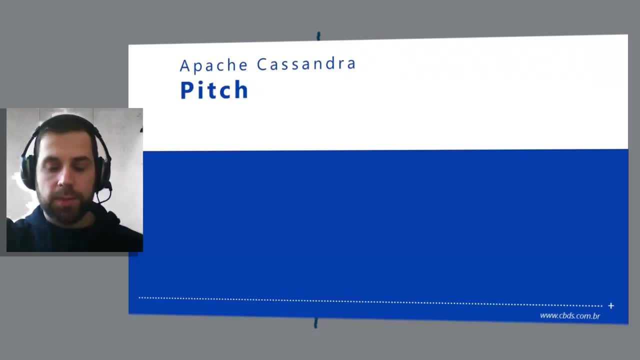 of the answer, Cassandra Peaches: Elastic scalability. Elastic scalability refers to a special property of horizontal scalability. It means that your cluster can seamlessly scale up and scale back down in an easy way. To do this, the cluster must be able to accept new nodes that can begin participating by getting a copy of 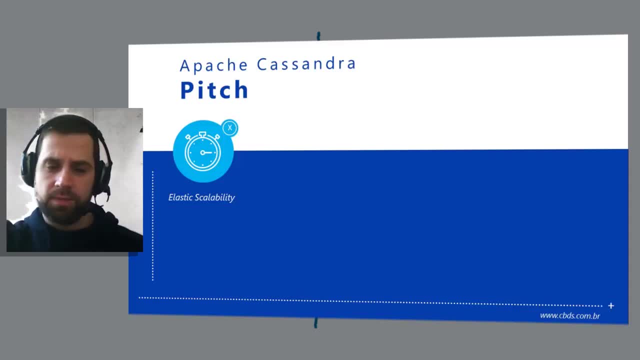 some or all of the data and start serving new user requests without a major disruption or reconfiguration on the entire cluster. You don't have to restart your process, you don't have to change your application queries, you don't have to manually rebalance the data yourself. 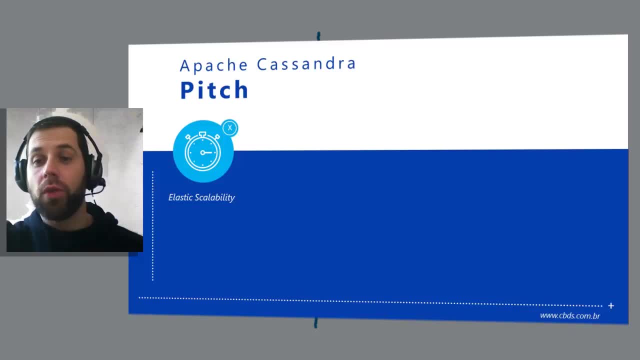 Just add another machine, Cassandra will find it and is starting sending it work. High Availability and Fault Tolerance. In general, architectural terms, the availability of a system is measured according to its ability to fulfill requests, but computers can experience all manner of failure, from hardware component failure, network disruption. 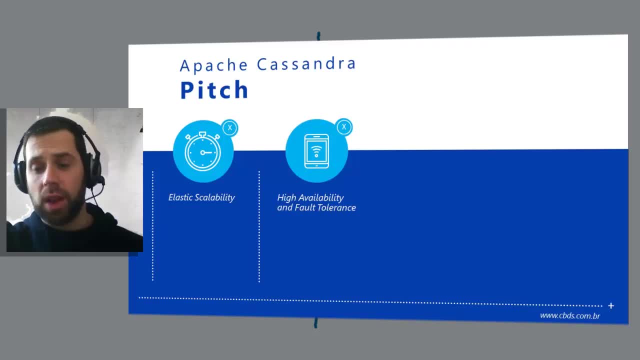 to corruption. Cassandra is highly available. You can replace, place failed nodes in the customer with no downtime, And you can replicate data to multiple data centers to offer improved local performance. Distributed and decentralized: Cassandra is distributed, which means that it's capable of running on multiple machines. 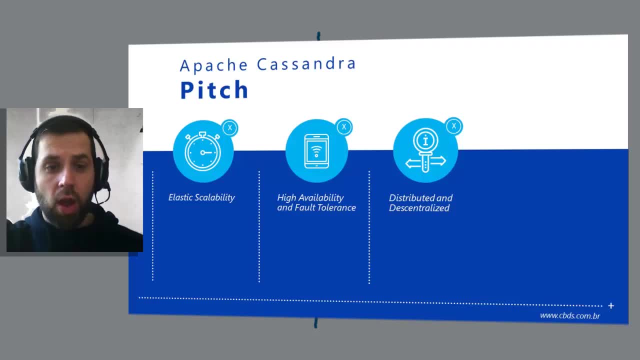 while appearing to user as a unified whole. On the other hand, once you start to scale many other data stores, like MySQL Bigtable, some nodes needed to be set up as master in order to organize other nodes which are set up as slaves. 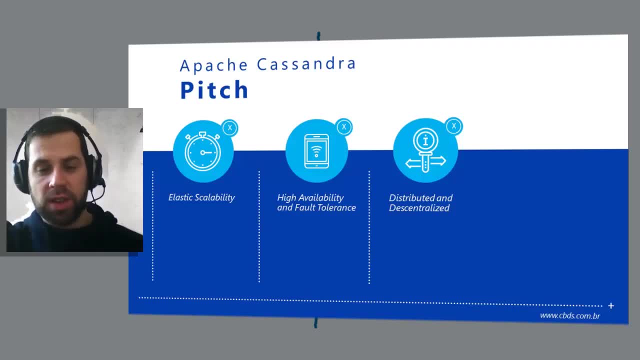 Cassandra, however, is decentralized, meaning that every node is identical. No, Cassandra node performs certain organizational operation distincting from any other node. Instead, Cassandra features a peer-to-peer protocol and use gossip to maintain and keeping sync a list of nodes that are alive or dead. 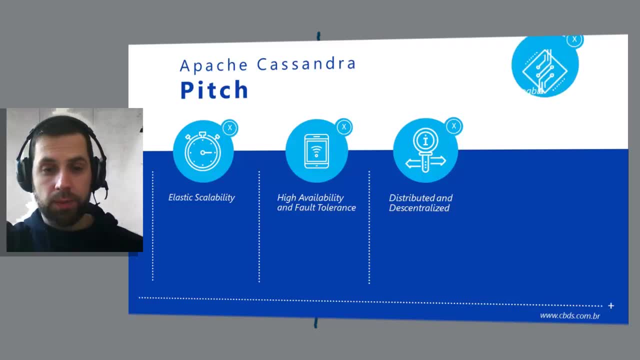 Decentralized means that there is no single point of failure. Turnable consistency. Consistency essentially means that read always return the most recently writing value. But there is no free lunch And, as we will see in next slide, scaling data stores means making search. 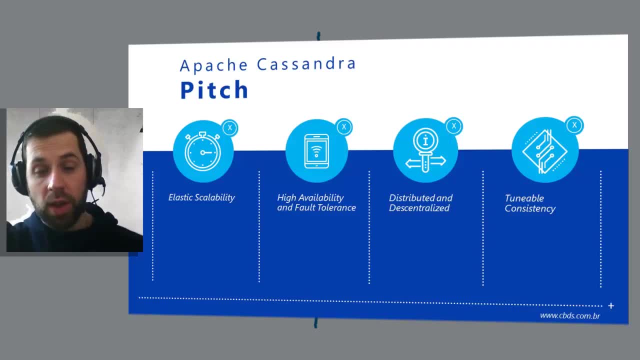 So I'm not sure you know what Cassandra is. The only way you can use Cassandra is by accepting trade-offs between data consistency, node availability and partition tolerances. Cassandra is frequently called Eventually Consistent Out of the box. Cassandra is more accurately termed 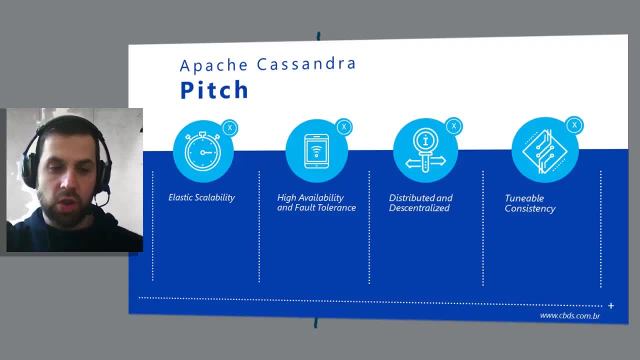 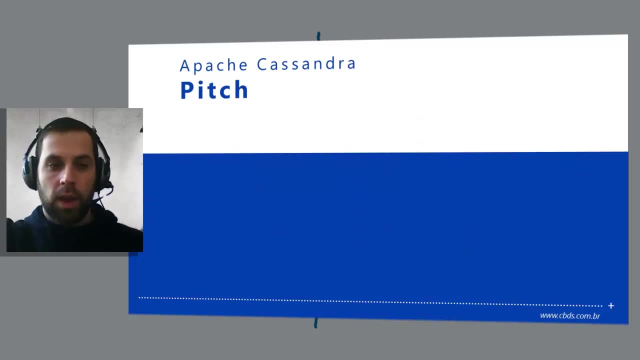 Turnable Consistency. Consistent, which means it allows you to easily decide the level of consistent you require in balance with the level of availability. Cassandra- Peach. Let's just see other features, other important features about Cassandra. The first CAP theorem. The theorem states that within a large scale, distributed data systems 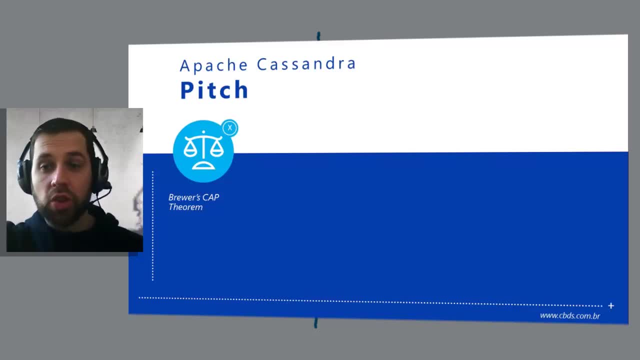 There are three requirements that have relationships: sliding: dependency, Consistency, availability and partition tolerance. CAP Consistency: all database clients will read the same value for the same query, even give you concurrent updates. Availability: all database clients will always be able to read and write data. 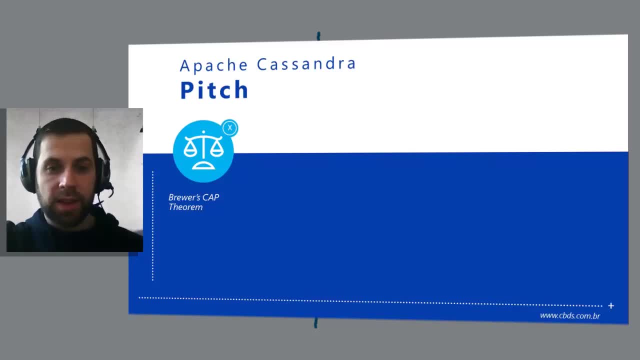 Partition tolerance. the database can be split into multiple machine. It can continue functioning in the face of network segmentation breaks. In a given system. you can strongly support only two of the three. We have to choose between them. because of this sliding mutual dependency, The more consistency you demand for your system. 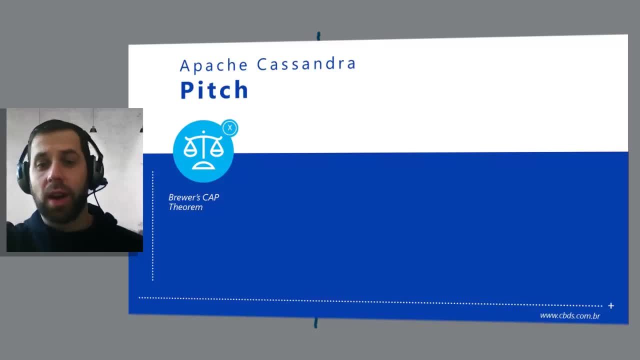 For example, the less partition tolerance you are likely to be able to make it, unless you make some concessions around availability. Row oriented Cassandra is frequently referred to as a column oriented database, which is not incorrect. It's not relational and it does represent its data structure in sparse. 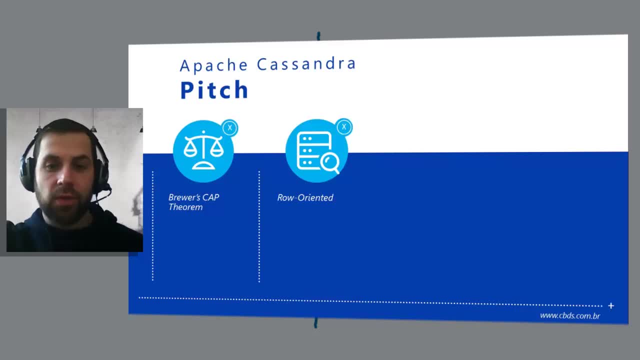 multidimensional hash tables. Sparse means that for any given row you can have one or more columns, But each row doesn't need to have all the same columns as other rows. like relational database models, Each row has a unique key which make its data accessible. Schema 3: 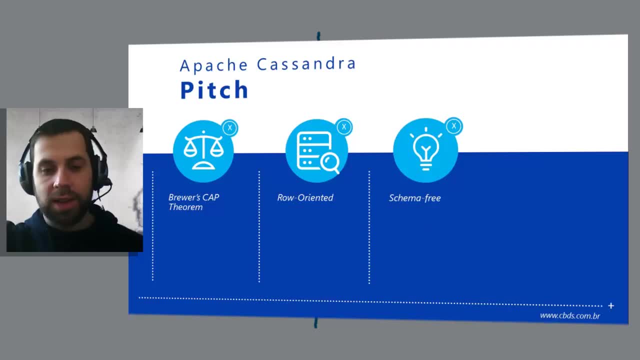 Cassandra requires that you define a container called key space That contains column families and certain configuration properties. the data table are Sparse. the data tables are sparse, so you can just start Adding data to it using columns that you want. There is no need to define your columns ahead of time. 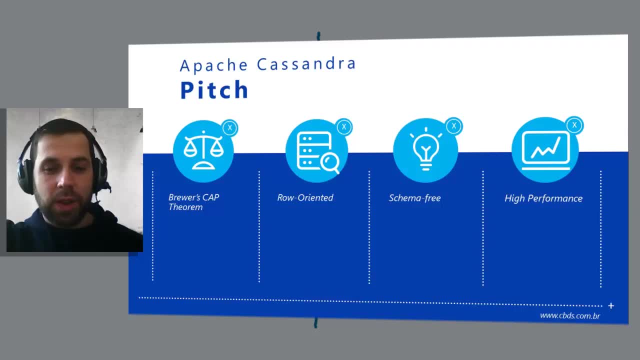 High performance. Cassandra was designed specifically from the Roundup to take full advantage of multiprocessor and multi-core machines and To run across many dozen of these machines Housed in multiple data centers. it scale consistency consistently and seamlessly to hundreds of Terabytes. Cassandra performed exceptionally well under heavy will, under heavy load. 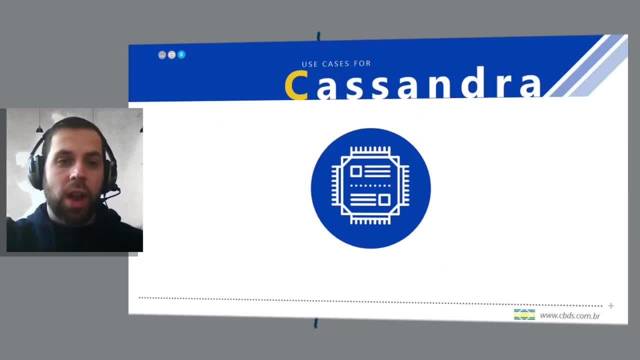 Use the cases for Cassandra. we have now an understanding of What Cassandra's advantage, so in this slide Let's take a quick look at what kind of projects Cassandra is a good fit. Large deployments: you probably don't drive a truck to pick up your dry cleaning trucks. 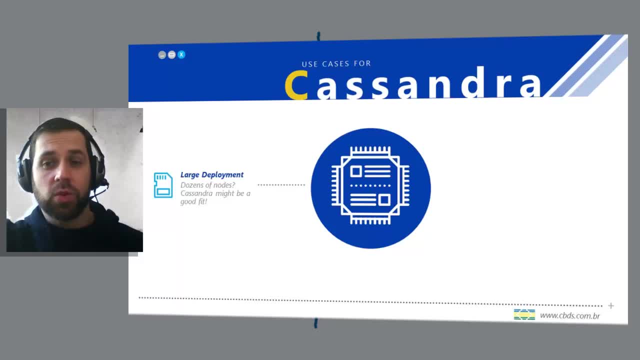 Are aren't well suited for that task, as we saw: Cassandra delivery, high availability, turnable co-systems, peer-to-peer protocol and see less scaling, but none of these Features is even meaningful in a single node deployments. There are, however, a wide variety of situations where a single node relational database is all we need. we may need: 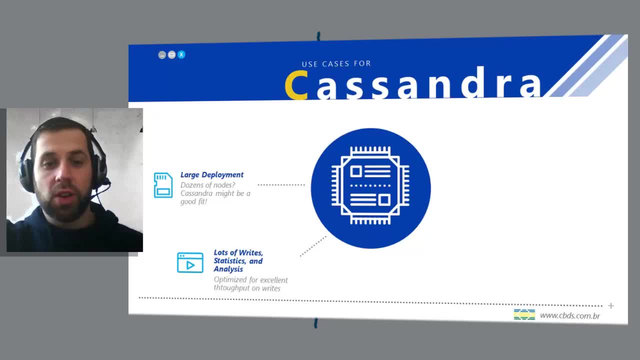 Considering your application from the perspective of the radio of reads. to write. Cassandra is optimized for excellent road put of rights. the ability to handle application workloads that require high performance at Significant right moments with many concurrent client threats is one of the primary features of Cassandra. If your application is 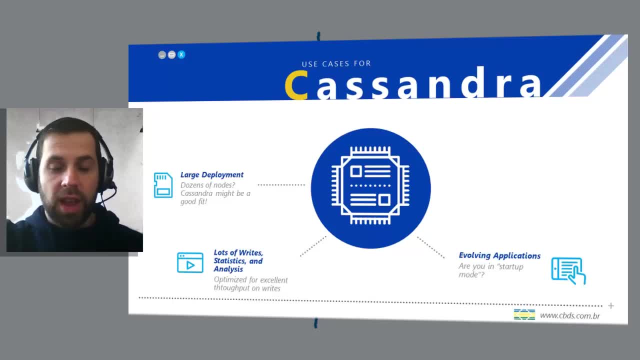 Evolving rapidly and you are in a startup mode, Cassandra might be a good fit, giving it a schema free data model. This makes it easy to keep your database in step with application changes as you rapidly deploy, and you can easily configure Cassandra to replicate data across multiple data centers if you have a globally deployed 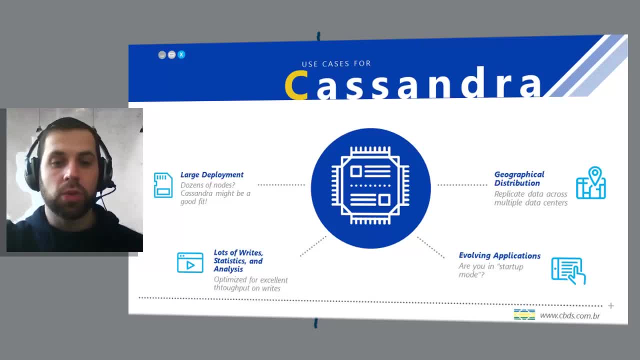 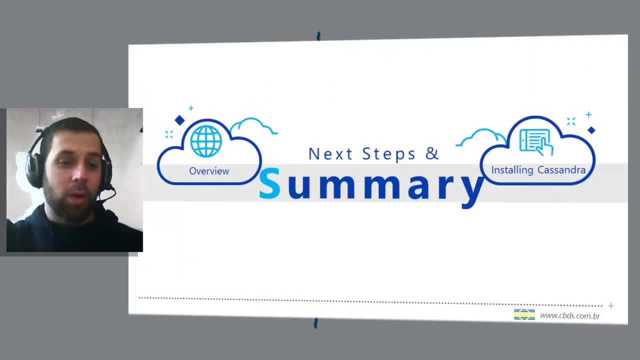 Application that could see a performance benefit from put the data near the user, Cassandra could be a great fit. Well, this is a short introduction about Cassandra. the next video- I will explain how to install Cassandra And use a CLI to interact with the data. so How do you you you when the next video will be available? 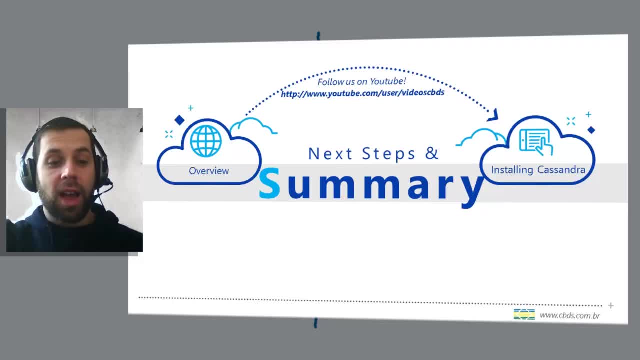 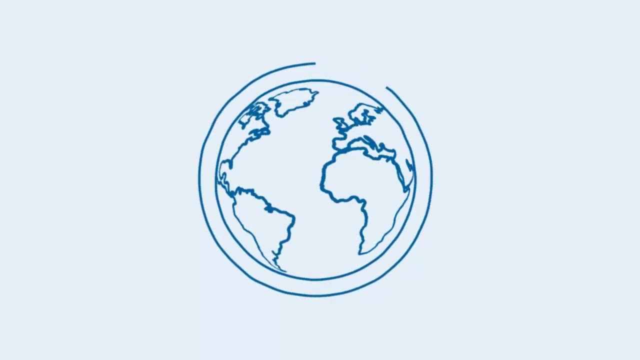 Follow us on YouTube. Finally, I would to thank your time And I hope that this video helped it to you learn more about Cassandra. See you, Bye, Bye You. 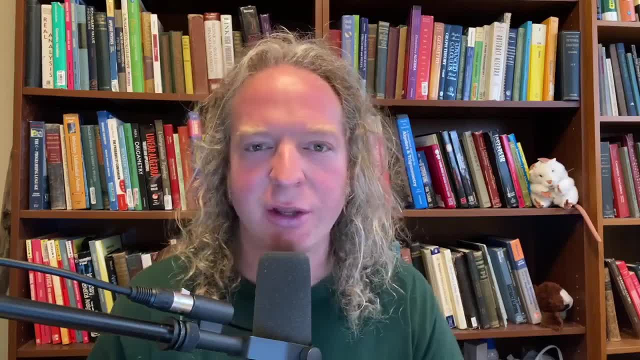 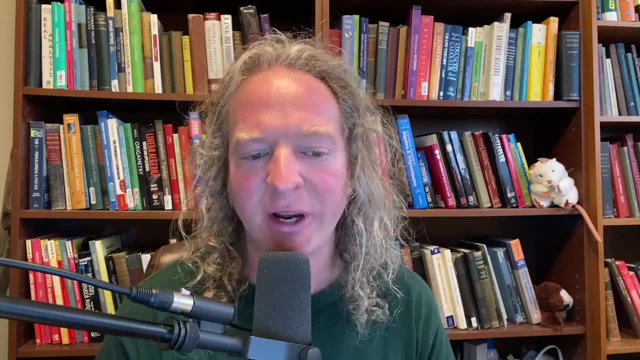 Hi, in this video I'm going to be answering a question that I received from a viewer. This person's name is Lindsay and the subject is worried about being unprepared for graduate school. I'm going to read the question in its entirety and then I will do my best to answer. 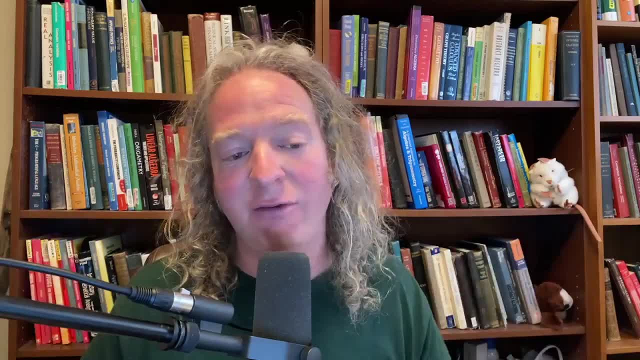 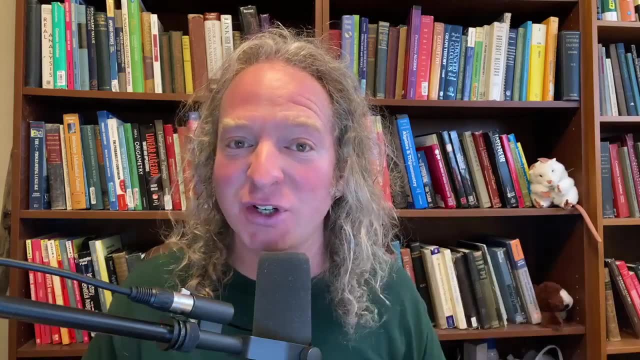 the question. I have not read this question yet. I've only read the subject and the person's name. so again, I'll do my best. If you have any advice for this person, please leave a comment in the comment section below. Remember, every time you leave a comment, it helps other people too. 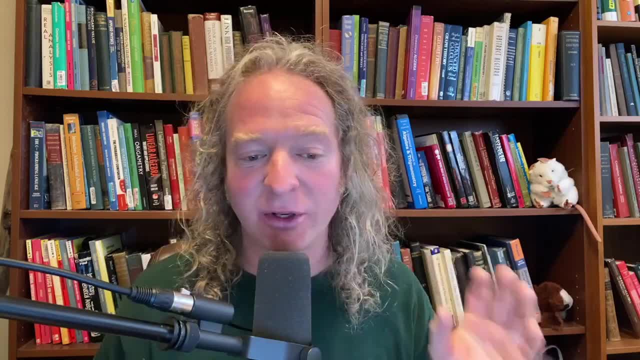 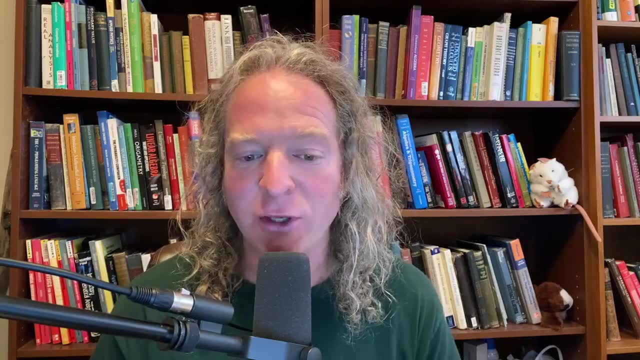 And this email seems to be very, very well written, so I'm going to go through it carefully and do my best. Good day, I've been watching your videos for quite some time and I was hoping that you might be able to provide me with some assistance. I received an offer for a master's 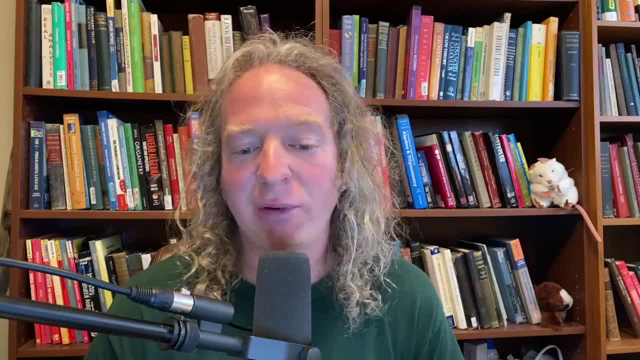 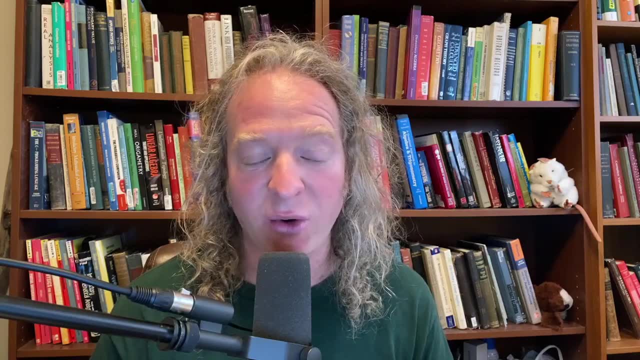 in applied mathematics at, and I'll leave the school out, where I plan on opting for the thesis option, where I plan on working with the financial mathematics research group To prepare myself for a career in quantitative finance. My concern is that, while I do really enjoy mathematics,